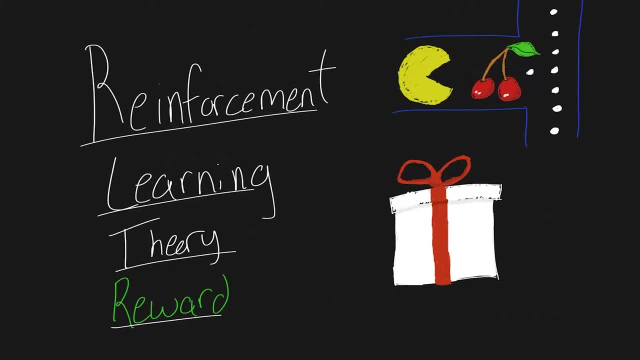 Hello and welcome. Welcome back to the Reinforcement Learning Theory tutorial series. This is part three of an ongoing series. You're more than welcome to start here if you want. If this, you just want to learn about reward and returns, But if you're interested in the rest, 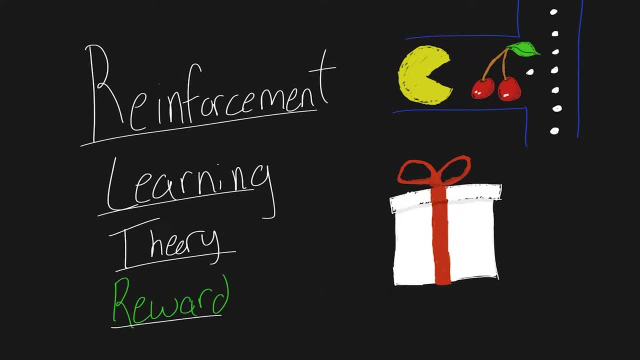 of it. it's going over general theory why algorithms work. what's going on under the hood, the math behind it, the theory, the intuition? definitely check out those videos. I'll have a playlist and such below As we go into the video, if you like, and the subscribe. 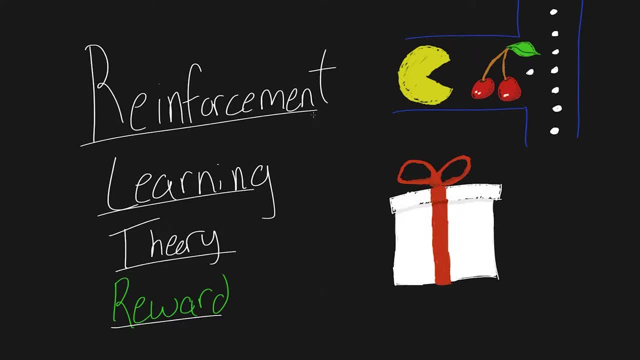 button really means a lot. But so much for that. That's enough of that, Let's get into it. I hope you like my little drawings. I'm not an artist, but I've been trying my best for you guys, So I hope you've been enjoying it. So, rewards, rewards- they're really important, especially. 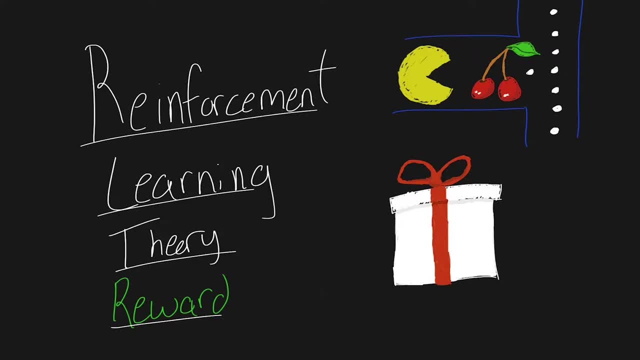 in reinforcement learning, where all our learning is, you know, based around rewards. So, as we're jumping into this, let me go ahead and get rid of this, so we have some space to work with As we talk about rewards. we're going to talk about rewards, So we're going to talk about rewards. 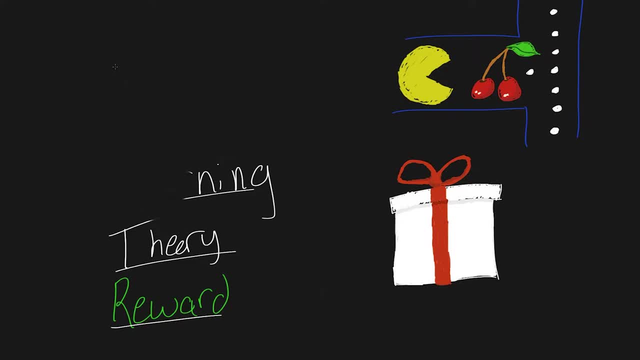 The first thing we need to talk about are returns, which are the rewards from trajectories, And I guess first, right, we should define trajectories. So what is a trajectory? And it's actually fairly simple. Remember back, we were talking about MDPs, markup, decision processes and environments and how. 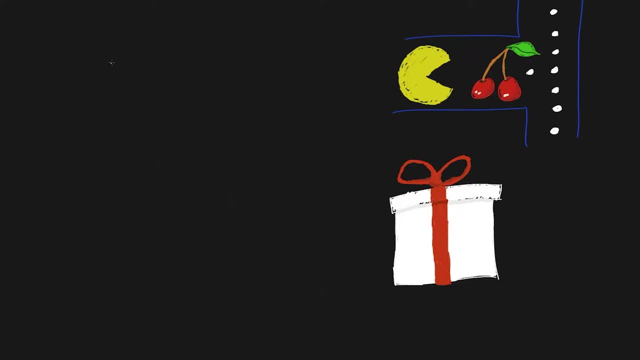 we would simulate environments right. So we had like a state space where we had a bunch of states like state zero, state one, and you know it goes on, And then an action space where we could have action one, action two, action three. These are all different actions. We 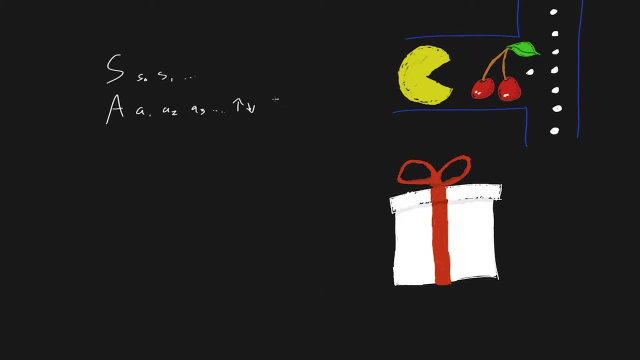 could take. you know it might be up down or it could be 3.4.. You know these could have different values and states. might be like the state of a tic-tac-toe game, like a circle in the middle. This would be one state. Well, a trajectory is very simple. It's sort of a: 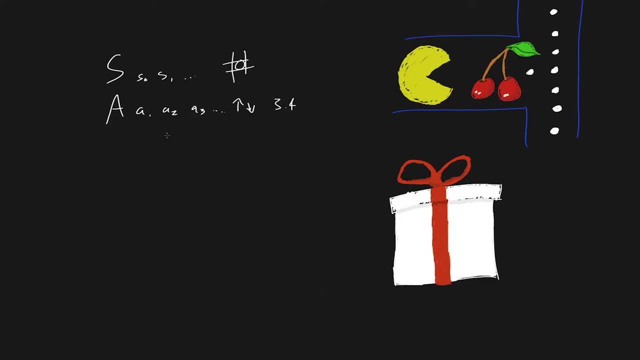 playthrough of a simulation, the history of one of these simulations or one of these playthroughs of a game, or the environment, So a trajectory, often one way we you'll see it denoted is: oh, that's not very good a tau. 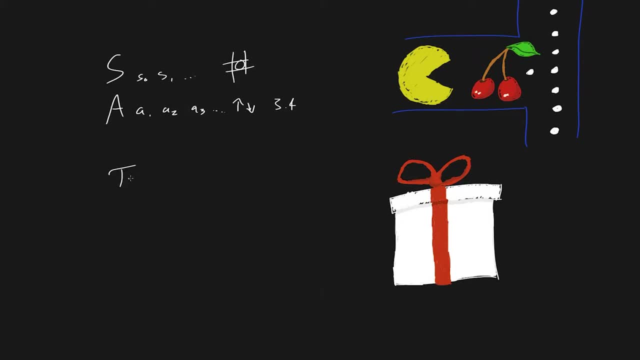 My tau is very bad. As you can see, I've not practiced drawing tau. Maybe if I make a little bit, okay I'll take it. I'll take it. So tau it's a little T thing And tau is short for. 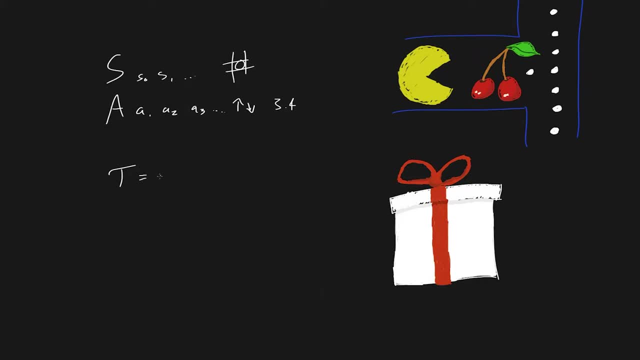 trajectory, kind of. Anyway, this will equal. generally, the way this is represented is: it's a state and then the following action that was taken in that state, the resulting state, the action that was taken in that state, then the next state action taken in that state, And you. 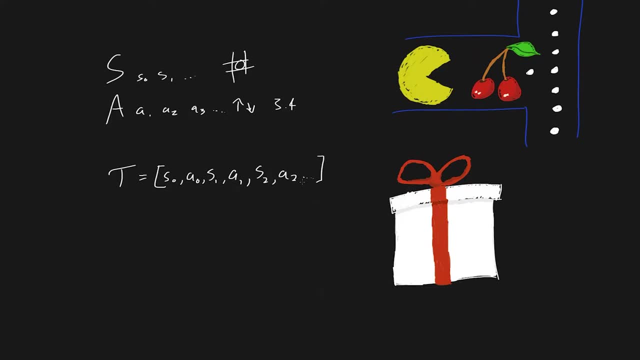 can see where this is going right, And this goes until the end of a simulation and a simulation right One full go through of the simulation. That is what a trajectory is And this is sort of the history of it. right, The states and actions, specifically, 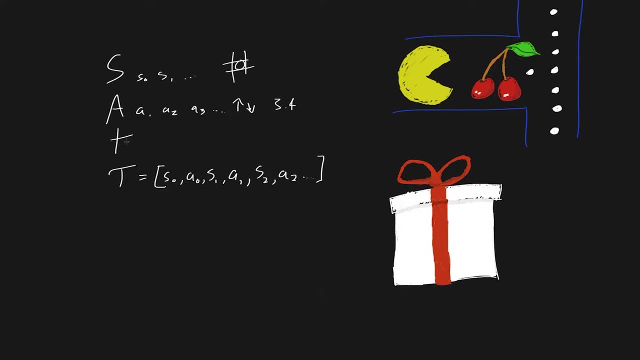 Cool, So not too hard right. Trajectories- So let me write that out: Trajectory: You'll also very commonly hear rollouts, roll outs, And the last thing you'll probably hear- maybe you'll hear more, But is an episode. An episode, I think, is what's most common. It's at least what I use most. 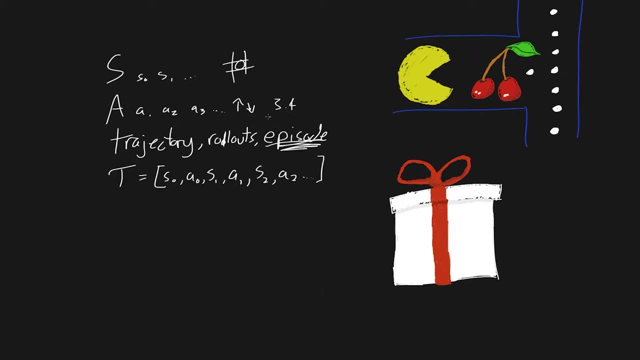 frequently. But you know you'll hear all these kind of interchangeably And they all roughly mean the same thing. So that's what a trajectory or like an episode is. So what about this term I mentioned before, A return right And a return? this is actually fairly simple. We have the idea. 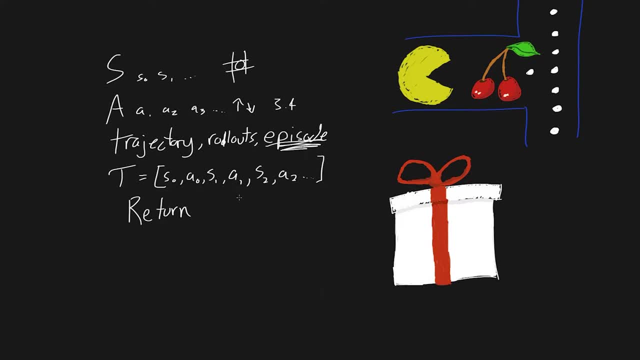 of rewards right, Like a reward could be positive for something And a return could be negative for something good, negative for something bad, Or maybe it doesn't have to be negative but just smaller than what you would get for something good happening. So the return is sort of the. 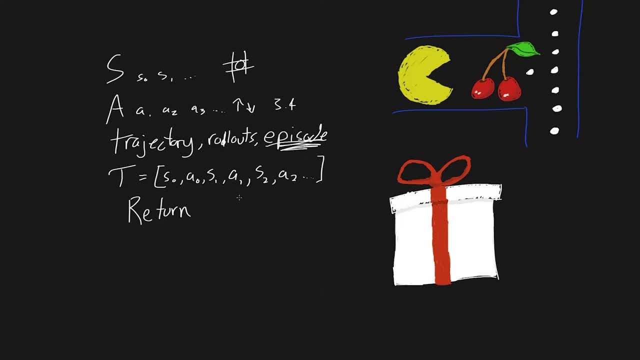 cumulative reward throughout a trajectory right. So let's say we're playing tic-tac-toe and we have, we end up in this right: X, X, X, O, O. Let's say we end up with a state like this: X is when. 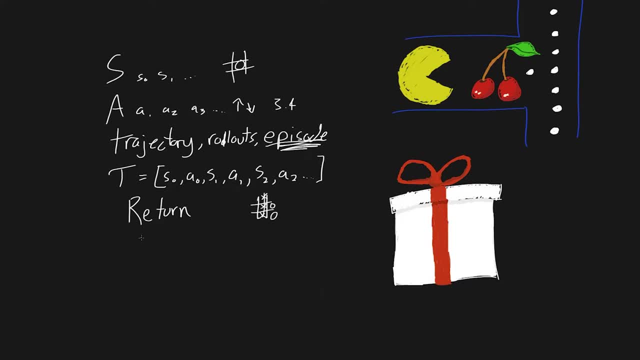 so if we were Xs- and this is like three turns long, right, Maybe our first reward, our rewards- maybe at first we get a zero for this first one because it's not doing anything, Then we get another zero because it's not doing anything, But then we put. 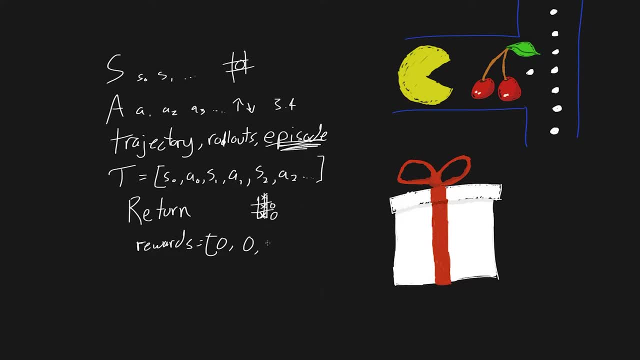 our third X here. And well, what do you know? We won the game, So maybe we get one reward for that. So these would be our three rewards for the game. So in this case, one way we could calculate the return would be zero plus zero plus one equals a one. 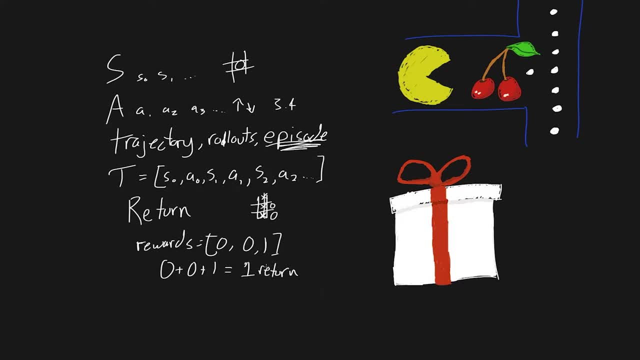 Return. This is one way to calculate returns, And this is what's referred to as a finite horizon, Horizon, Undiscounted, Undiscounted return. And let me make some more space for us. Oh, took me so long to draw this present. It's so bad, though. Anyway, we have more space to work with. 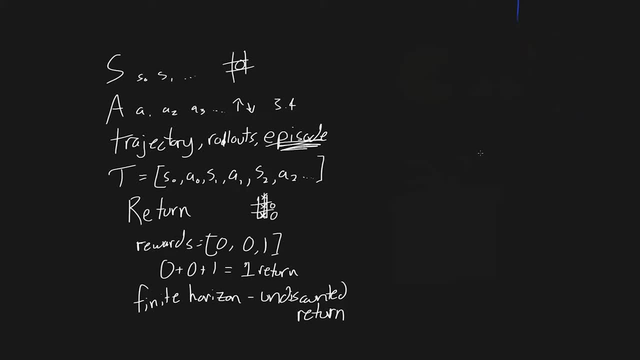 now. So that's an undiscounted return, And then we have a finite horizon, And then we have a finite return. Why is it discounted Undiscounted? What that essentially means is that, no matter how far after or how far away this reward is right, It's always counted as one, Whereas with it sorry. 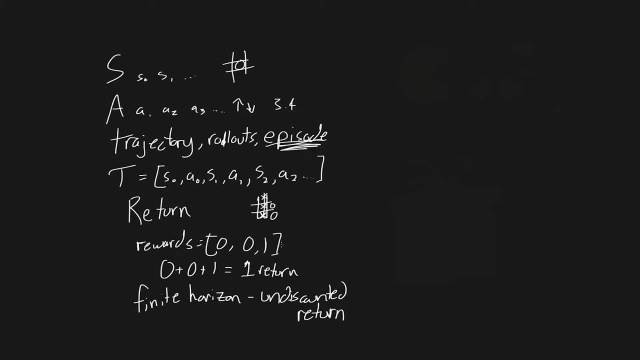 not as one. It's always counted, no matter when it happened, So long as it happened after the current time. And when we're talking about returns, we're talking about the whole course of this right, But oftentimes we'll be talking about rewards from a certain amount of time. So 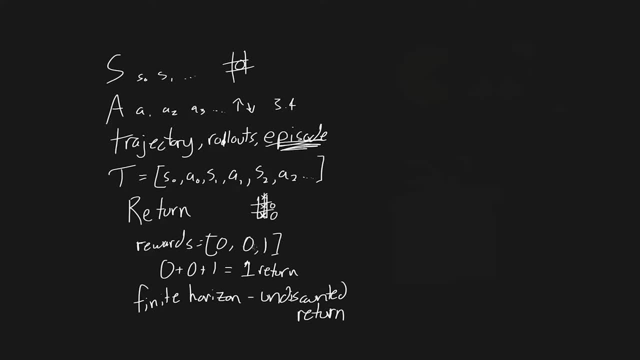 say from the second state. So the cumulative return coming from the second state, everything after this would also be one. I mean the same for the third state. But you can imagine let's get a little bit more complicated reward here, Or a series of rewards. So we have one, two, zero, five. 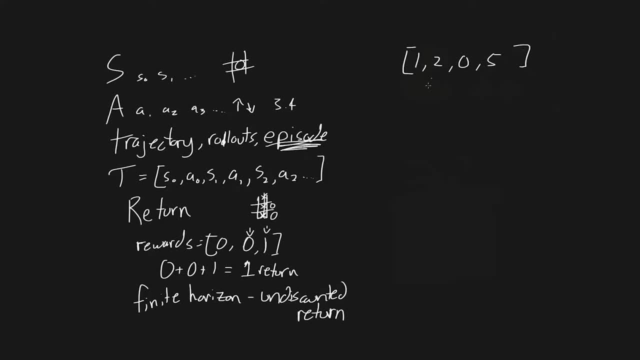 So let's say we have something like this, right? Well, in this case, our total return for this episode would be eight. We just sum it all together, Okay, But what if we're in this state? right here, If we are in state, we'll call this state zero one. 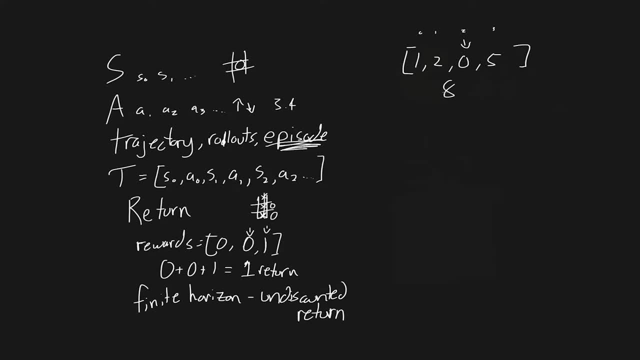 two, three. So if we're in state two, well, what's our return for coming from state two? And sometimes this is called the value, or it's always called the value. Well, it's five, right, Only five. 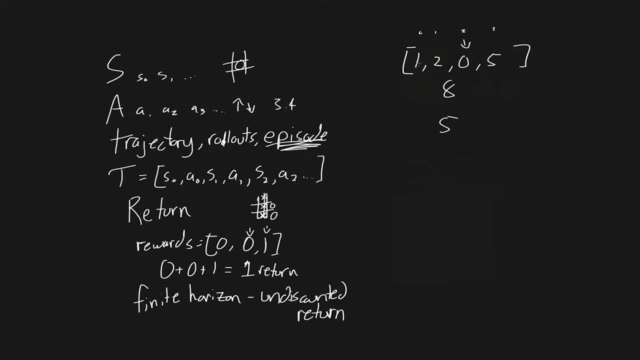 because we're not going to get the one and two that already happened. We're not thinking about the past at this point, So we'll move on to the value in the future. But I mentioned this right now because It kind of makes sense to mention this, with undiscounted and discounted returns, because 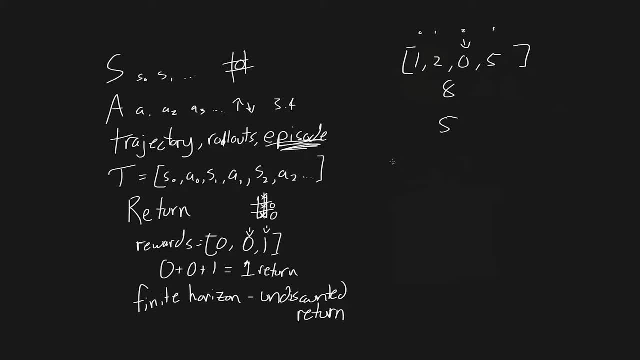 now I want to tell you what a discounted return is. A discounted return is specifically in What is it? This was a finite horizon, So next is an infinite horizon- discounted return. So what's this? And this is essentially the idea that 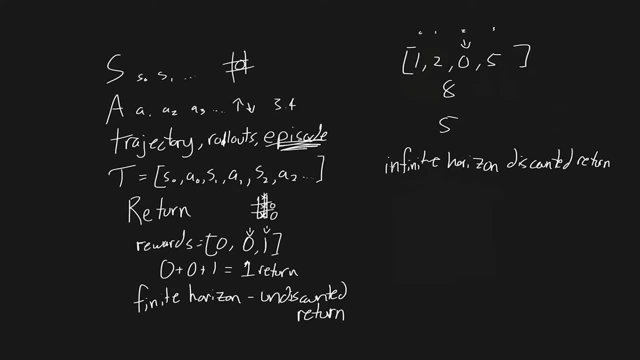 idea behind it, at least versus what I want to go over, and the intuitive idea is that if you get a reward for doing something immediately, that should be more important than a reward that happened, say, 10 steps down the line or a million steps down the line. right, there's sort of a good part of 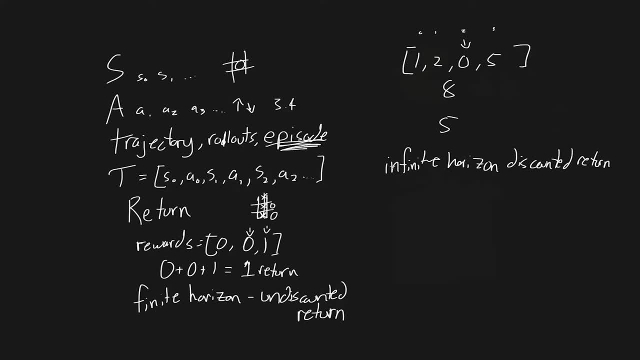 getting something done now. now, whether or not we should be using discounted reward, that's another question. I'll talk about sort of when we use it and when we don't want to use it. but the mathematical formula for it is something like this: right, so we want to have a, and I'll I. 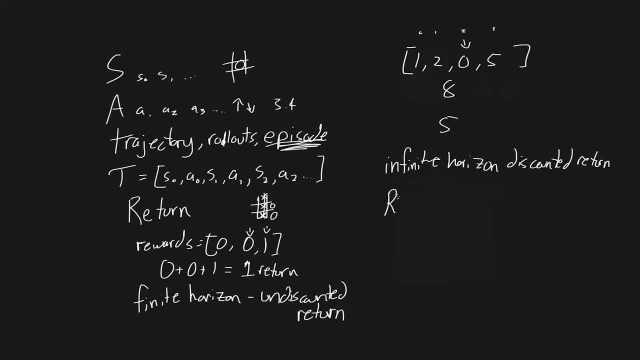 guess I should write out what it equals first, right? so the return, often denoted by a capital r of a trajectory equals the summation to infinity, starting from the first state of r of t, zero, zero times gamma. to the t. what is this gamma? that is a good question. this is our discount factor. 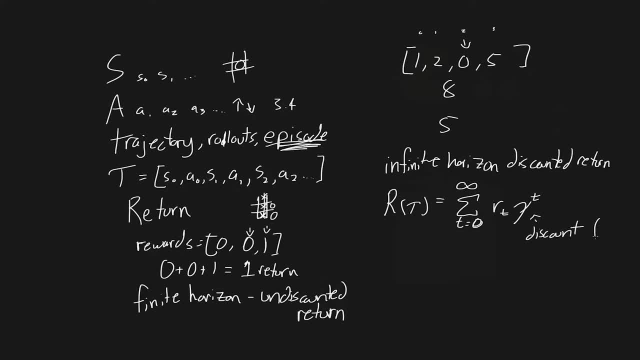 so this is called a discount factor factor and it's usually equal somewhere between zero and one, or always equal to somewhere between zero or one. and essentially what this means, right is it means in the very first step, the very first time step, so let's say, let's say we're just, let's go back. 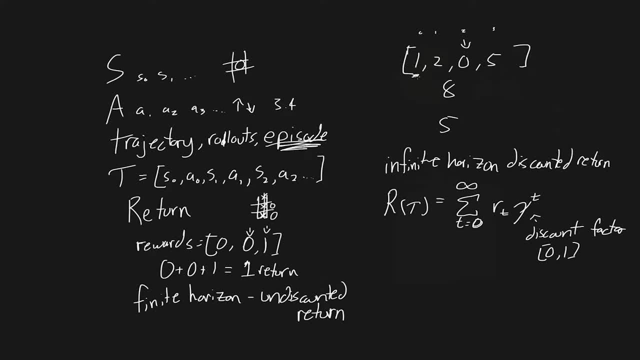 to the idea of taking whole trajectories right. so we're starting from the first state here with this one, this one reward. well, in this state we get a one reward right. so this will be one reward plus and, let's say, our gamma is equal to 0.5. 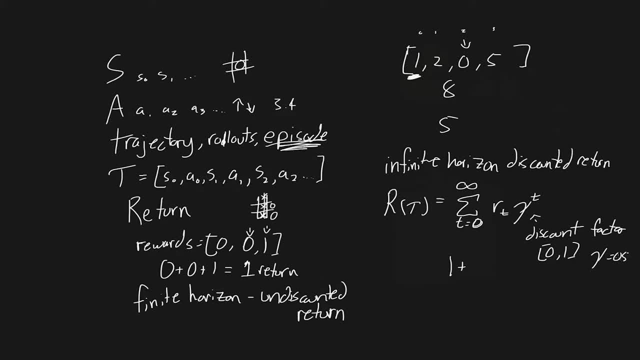 say, gamma equals 0.5. sorry, that's on the edge of the screen. what would that mean? so it would mean, well, t to the 0.5, to the zero, that's still one. so we start with one. two is our next reward, right two. 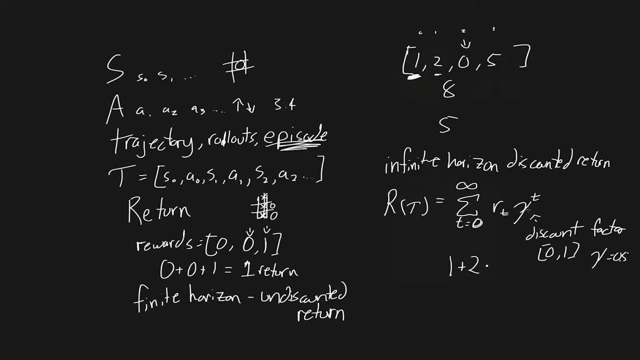 times well, this would be what? 0.5 to the 1 times 0.5. so this gives us 1 plus 1 plus. uh, well, this is a 0 plus and then finally 5. so it's 5 times gamma. 0.5 to the 0, 1, 2, 3. what would this be? that'd. 5 times 0.125, which i don't really know how to do. so we start with, and then we just: this means like well, it would be like a very high, and so this one, let's just let us do this. so we start with gz: equals for z. so the first let's just take gz, and so this gives us r right, and so let's say 0.05 of this. dash is equal to one plus 1 plus 1 plus. so let's say gz equals 0.25, so this would be 0.05. so this comes out to the whether this is 1 plus 1 or it's the same thing, because we already know this. 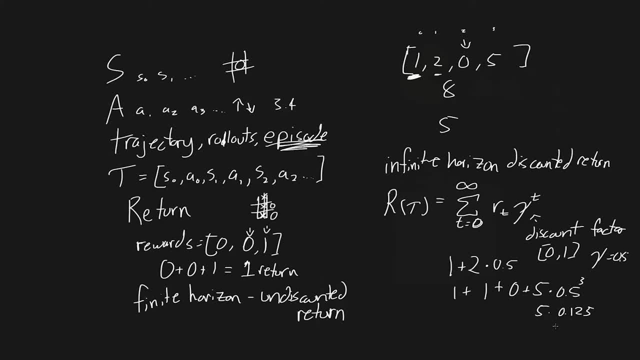 which I don't know what that is, or I guess it would be like 0.6 something, I think, if I'm doing my math right, yeah, So essentially what I wanna show you is, at the very first state, here we have the full reward. 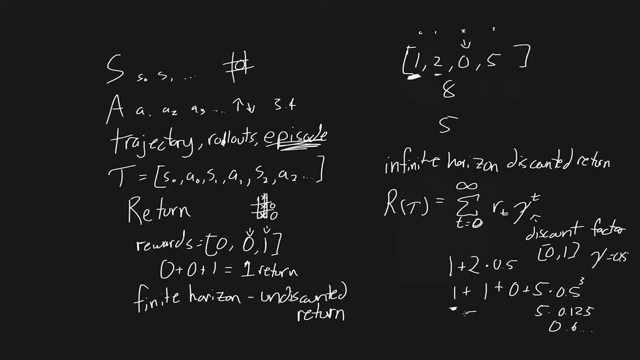 The full reward was one. We're counting it fully, but as we go down and as time progresses, well, by the end here, even though there's a five reward, at the end, it's only being counted for 0.6.. 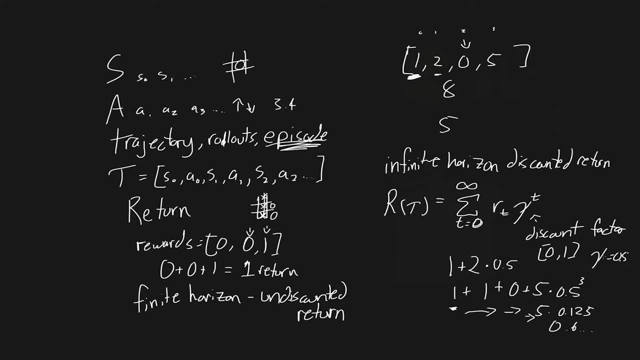 So, essentially, the higher gamma is, the less important things in the future become and the more we prioritize things now. That's sort of the intuitive meaning behind this. So, comparatively, if we want to- and I'm gonna- oh gosh, what should I erase? 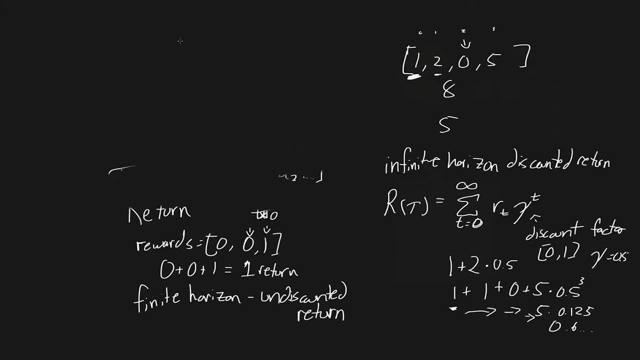 I'm gonna erase some of this because we need more space. Oh no, why does it keep doing that? I need to fix that, Anyway. so finite horizon, undiscounted returns- right, And this is also where the infinite and the finite comes in, right. 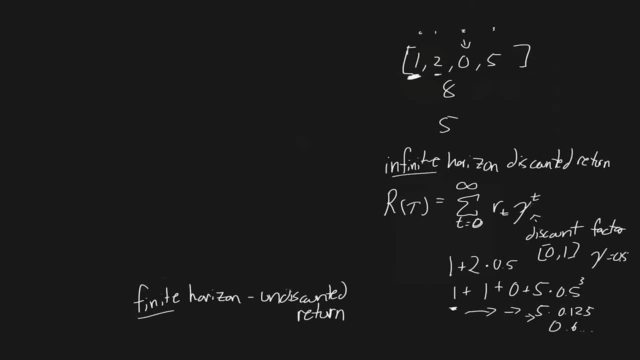 Infinite, as in this, can go on for infinity and it will still converge because of the fact that we have this gamma term here. And even if we go for infinity down the line, well, eventually gamma will get so small that all rewards are just negated. 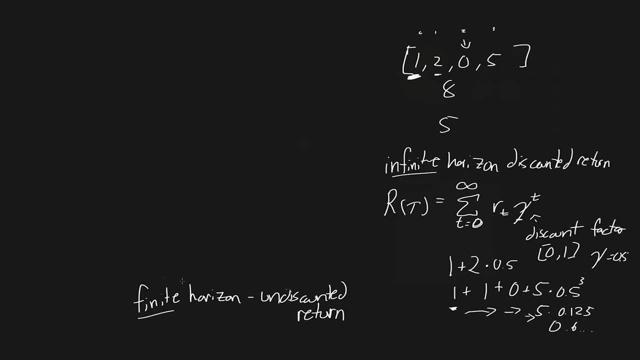 Whereas for finite we can only deal with a finite amount of space, And this is really in terms of mathematical algorithms we come up with down the line For finite or for undiscounted returns. we can't really handle infinite series. Things just get a bit wacky with math. 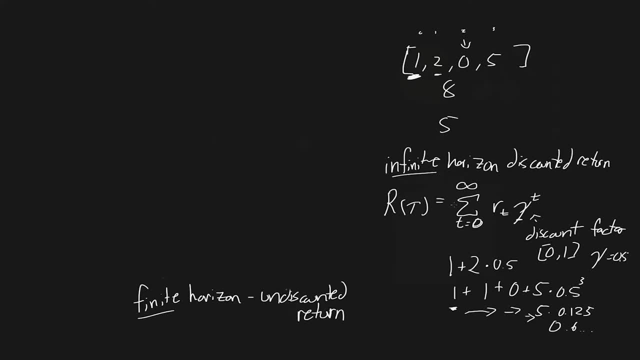 Maybe we'll get more into that when we get into specific algorithms, But for now, the reason we do this- can be infinite- is it just ends up being more mathematically convenient. So the equation that I was gonna mention for finite horizon is the return. sorry, 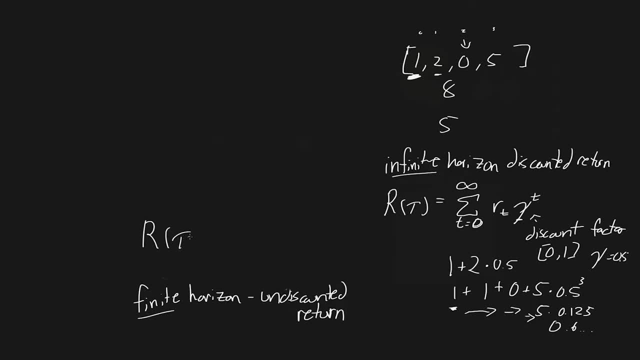 of the trajectory for finite equals. I guess it would be: t equals zero to capital T. So this is some point in the future of R of t, Very simple right. So it's essentially just a summation over all the reward over the next t steps. 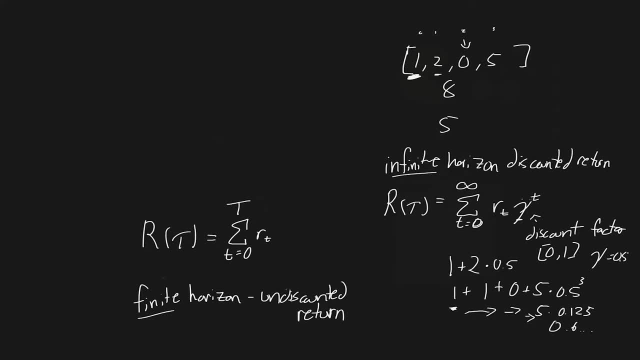 So the only difference here really is the infinite versus the finite and the gamma versus the no gamma. So the answer is no today or no scaling Cool. So you know it's not too complicated. I think the intuition behind it makes a fair bit of sense. 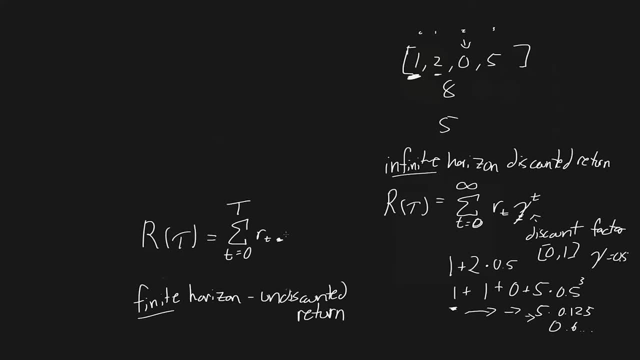 Generally, we do want to prioritize things immediately a bit more, Though things in the future are important too. Well, the value of gamma sort of lets us decide how much we want to balance this. So one question you're probably asking is: well, what value should I use for gamma? 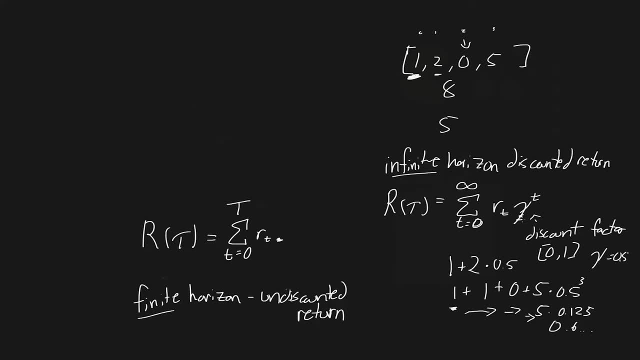 What's normal? And the answer is: it depends. It depends on the environment, but there have been lots of studies that say well, lots of studies that show gamma usually around the range of oh gosh, I'm running out of room again. 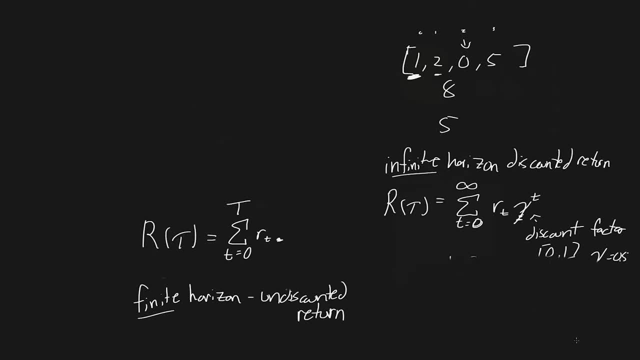 um, let's just delete this example right here. um, usually, so usually, it's always within the range of zero to one, but usually within the range of 0.95, and 0.99 are probably what you'll see most frequently. uh, and I hope that's big enough I can erase, just in case. um, but 0.95 and 0.99. 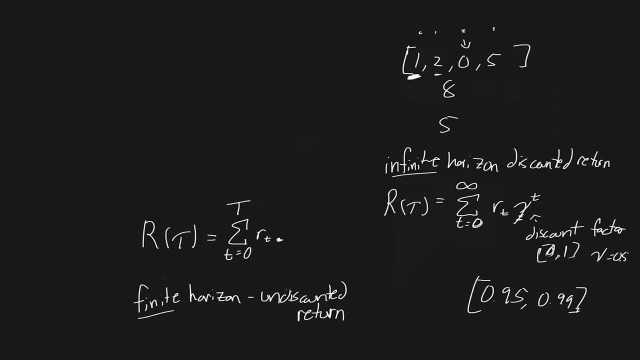 are the most frequent, um, so you can see, these still do, uh, value actions in the future quite a bit. uh, we don't want to completely disregard them because they are very important uh, but yeah, that's what you'll usually see. so the next question you might be asking is: well, you know, we have 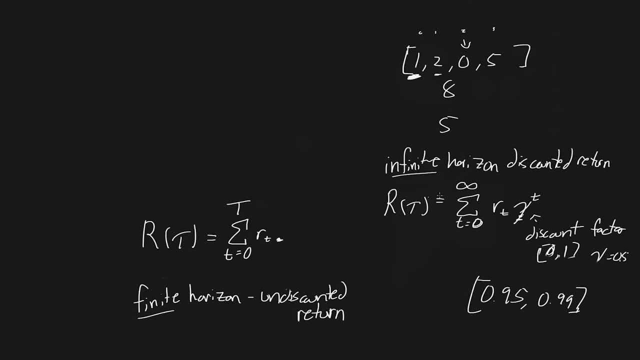 finite horizon undiscounted rewards and we have infinite horizon discounted rewards. but which one should I use? and, and unsurprisingly, the answer is again: it depends. uh, that being said, there are some sort of pointers you can use. I tend to see discounted returns used in the majority of 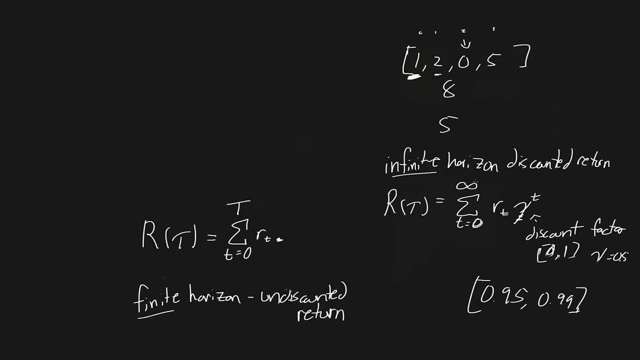 things because, especially in games where you have a lot of rewards throughout, um, but in games where you tend to have maybe one reward at the very end of a of a episode, especially in things like board games, right, where it's like a winner or loss and that's your only reward- finite horizon rewards. 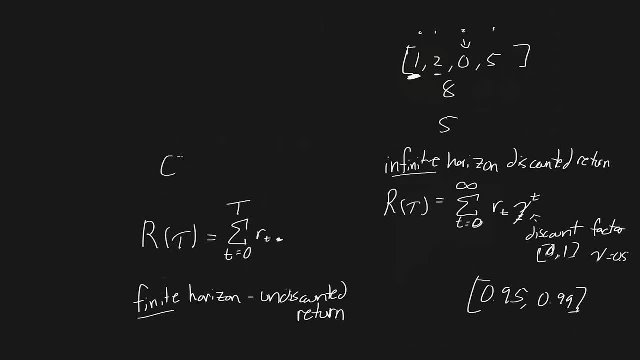 tend to be the most common one. so I think that's a good question. and I think that's a good question. I think that's a good point. if you're watching from the beginning of this video, you're probably used there more often, so like you'd probably see this in. like you if you're using chess or go um you. 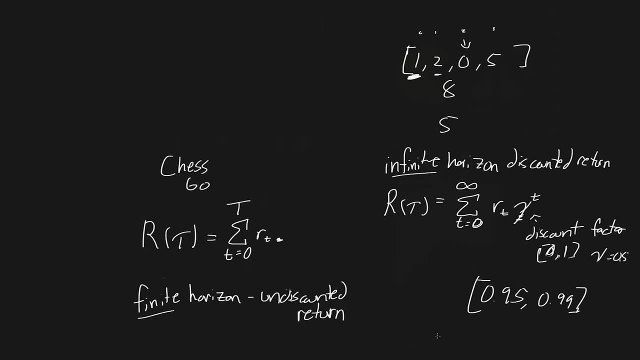 don't have to use it, um, but you'd see undis or sorry, discounted rewards in in environments more like, uh, maybe self-driving cars, driving cars because you know they go for a long time, um, you know, not infinite amounts of time, uh, but you know, and you, you also have these sorts of rewards that 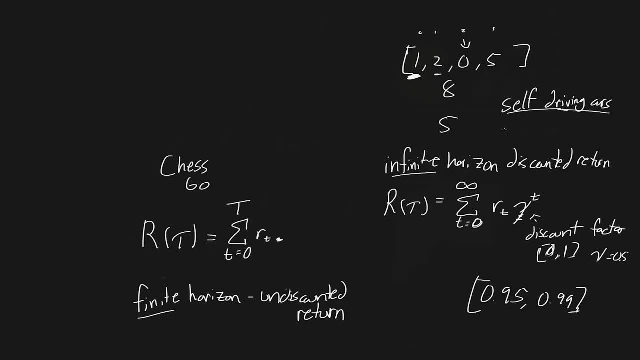 coming go. it's not just one big reward at the end. and also, like I said, the same thing you know when you're of games like atari. you know atari is a very, very popular environment to test machine learning or reinforcement learning algorithms specifically, and i think those are are sort of the big things that 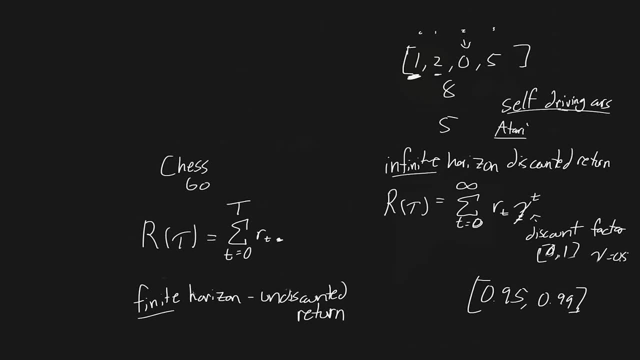 you should know. so just summarizing that finite horizon on discounted rewards, it's just the sum of rewards over a fixed time period, very commonly used when using board games or when you have one big reward at the end of a finite time series and the sort of other option is infinite horizon. 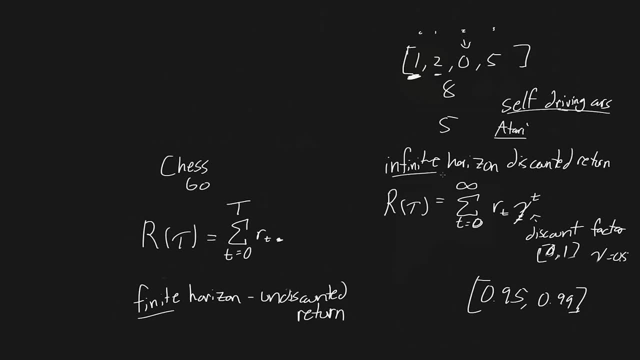 discounted returns and you see these in pretty much all the other scenarios where you have very long time spans you're working over and when you have also rewards throughout. i'm sort of coming and going and yeah, i think that sort of wraps up the key points of rewards and returns.